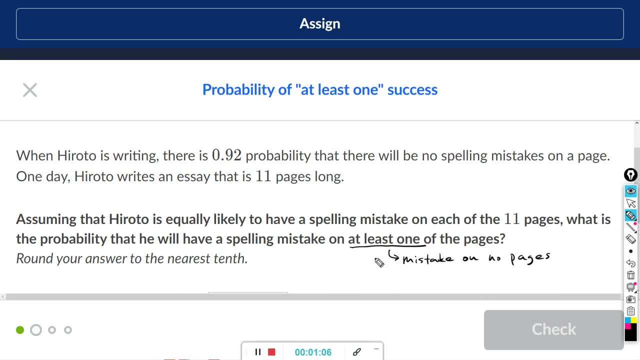 That's going to be the complement. Remember: for complement, we just subtract it from 100% or the number 1.. I'm going to do 1 minus the probability that he has a mistake on 0 pages. In other words, no mistakes. 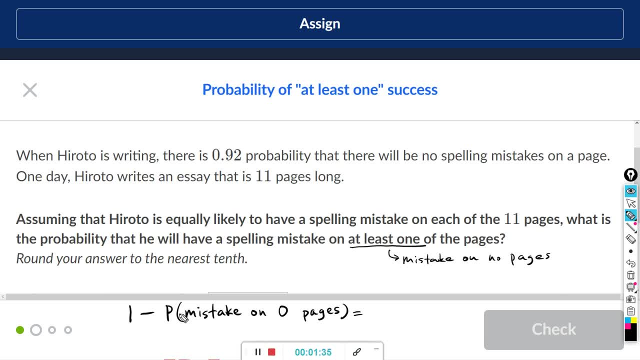 So we're starting with 1, or 100%, and we want to find the probability that he has no mistakes or a mistake on 0 pages. So it says there's a .92 probability there will be no spelling mistakes on one page. 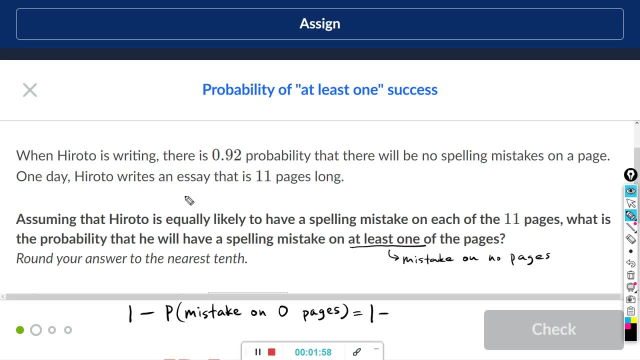 So for the first page, for the first page, the probability of no mistakes is .92.. And then on the second page, the probability of no mistakes is .92.. Okay, and so on, and so on. It keeps going, And we can just multiply those, because those are independent events. 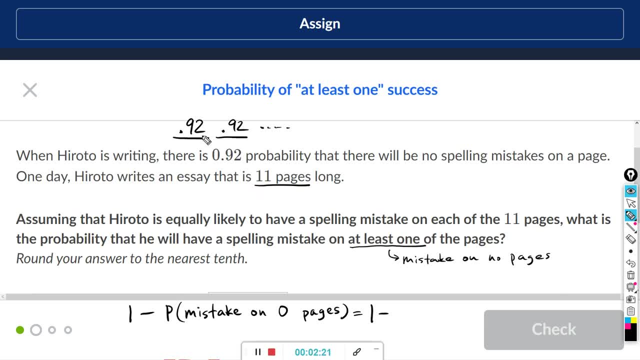 So for 11 pages it's going to be .92 multiplied 11 times. Alright, so it's just going to be .92 to the 11th power, 1 minus .92 to the 11th power. So we're just going to do that on the calculator. 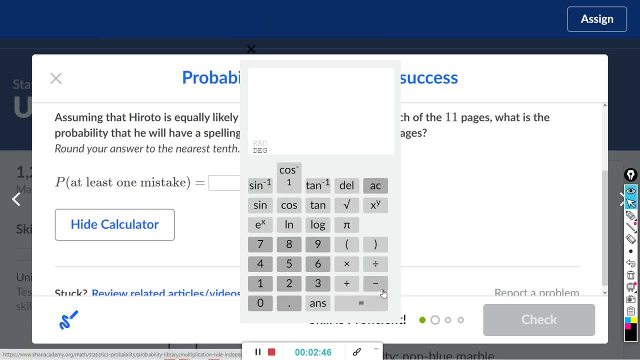 Okay, so I clicked show calculator, but of course you can use your own And I'm going to do 1 minus .92, and this is for the exponent right here, the x to the y button, And I'm going to make that to the 11th power. 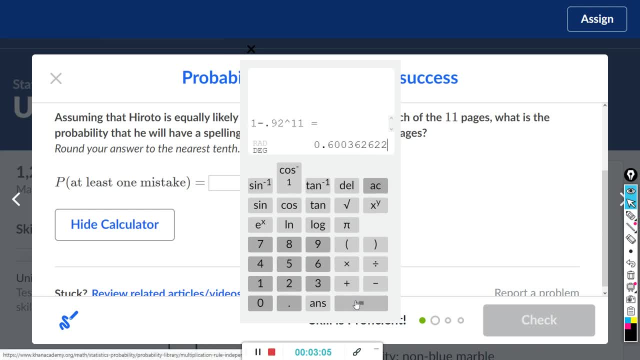 So it's 1 minus .92 to the 11th power. Okay, and when I hit equals, it's a pretty big decimal, But it says right here, round your answer to the nearest tenth. That's only one decimal. 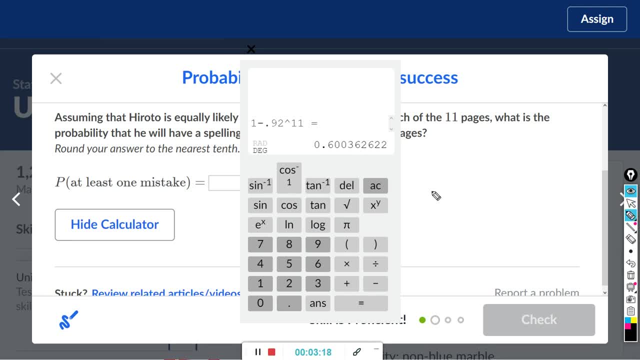 Okay. so in order to round to one decimal, you look at the second decimal. Okay, if it's 5,. if it's less than 5, you round it down. Of course, 0 is less than 5, so we're just going to round it down. 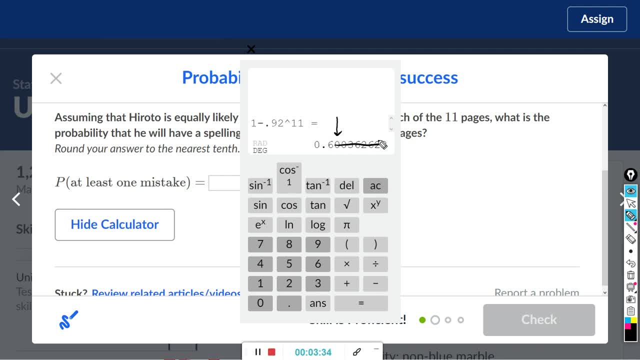 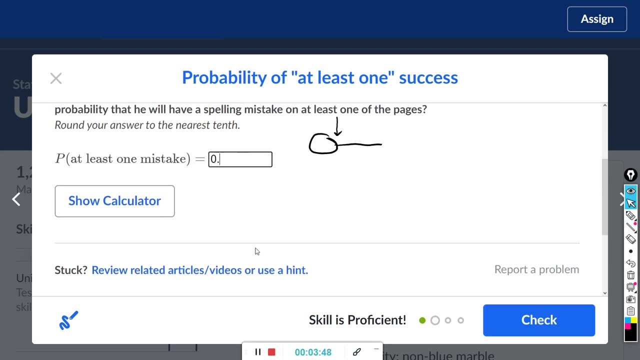 Alright. when I say round it down, that just means you eliminate the extra decimals. So this is the answer right here: 0.6.. So you just click in the box and type 0.6.. So inside the box: 0.6.. 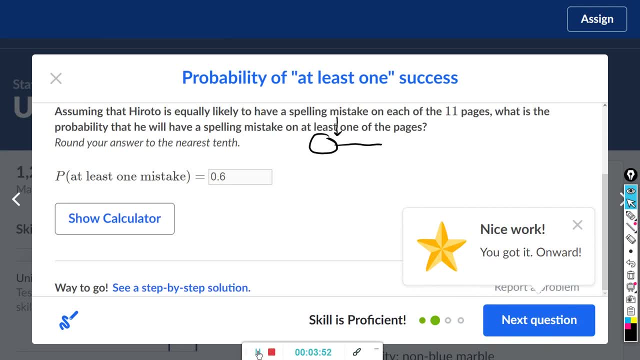 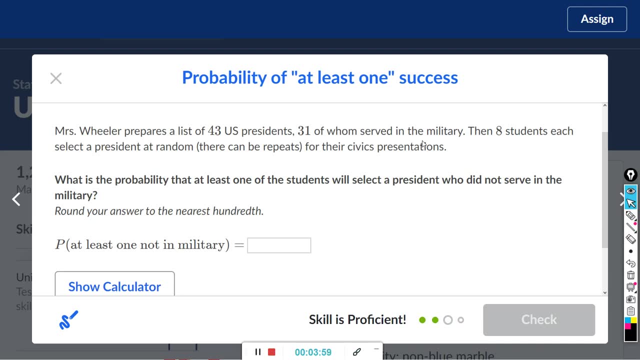 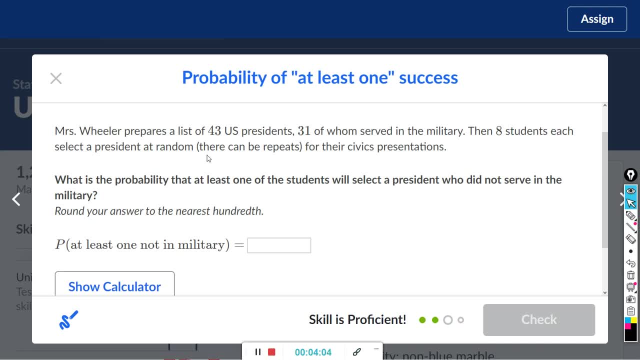 Then eight students each select a president at random. There can be repeats for their civics presentation. What is the probability that at least one of the students will select a president who did not serve in the military? Okay, Again, we're just going to do, since they said, at least one who did not serve in the military. 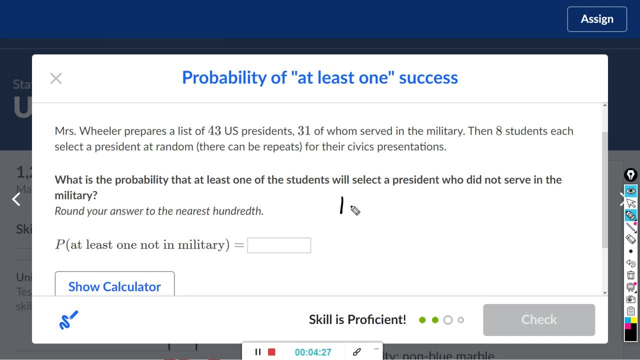 we're going to subtract the complement. So we're going to do one minus the probability that if it's going to be at least one who did not serve in the military, we're going to do one minus the probability that they all served in the military. 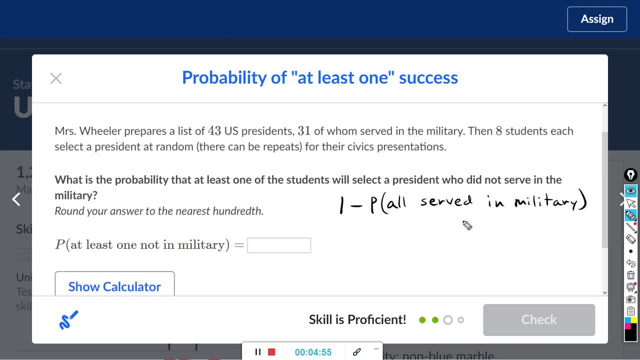 Okay, So that's the complement. Complement. So that's going to be one minus Okay. So let's see here. Remember that eight students are selecting, Okay, And there can be repeats. So the probability, The probability of one of them serving in the military. 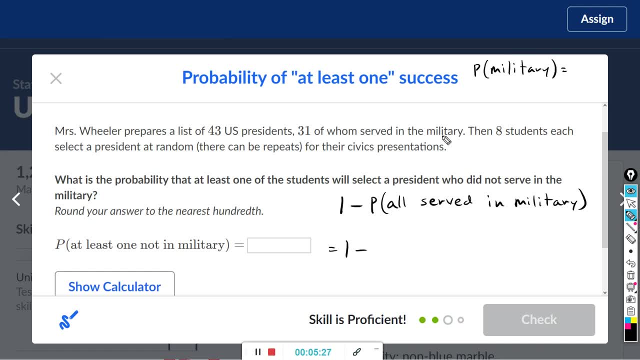 Since thirty-one out of forty-three served in the military, it's going to be thirty-one over forty-three, Okay, And remember, eight students are selecting, So we're going to have to multiply this eight times. Okay, It's going to be thirty-one out of forty-three for the first student selection. 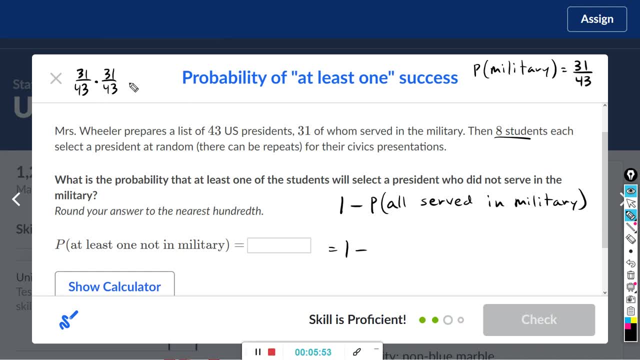 Then thirty-one out of forty-three for the second student, Okay, And so on. It just keeps going, And since eight students are selecting, it's going to get multiplied eight times, So it's going to be thirty-one out of forty-three to the eighth power. 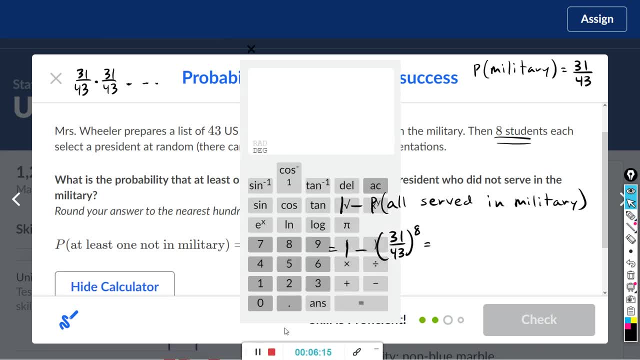 Alright. So it's going to be one minus thirty-one over forty-three to the eighth power. So on the calculator, one minus and use parentheses: thirty-one divided by forty-three, close the parentheses and that gets raised to the eighth power. 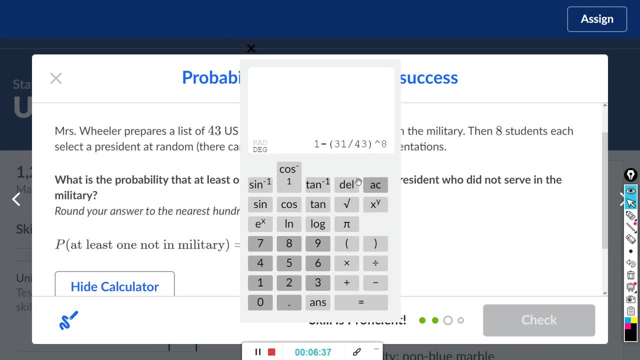 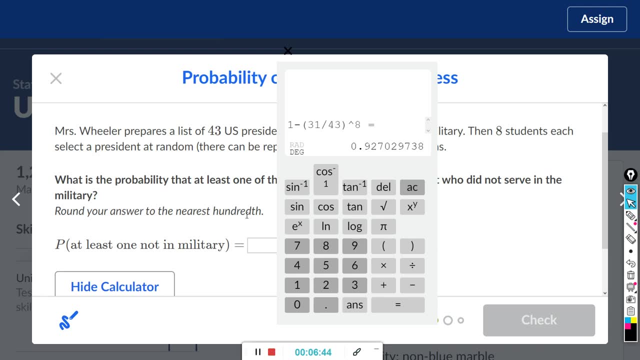 So you see that One minus thirty-one over forty-three to the eighth power I hit equals. It's a big decimal, Okay, But you can see here it says round to the nearest hundredth, That's two decimal places. So you want to go to the third decimal. 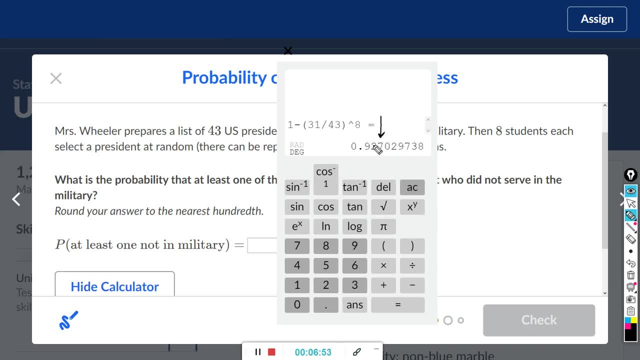 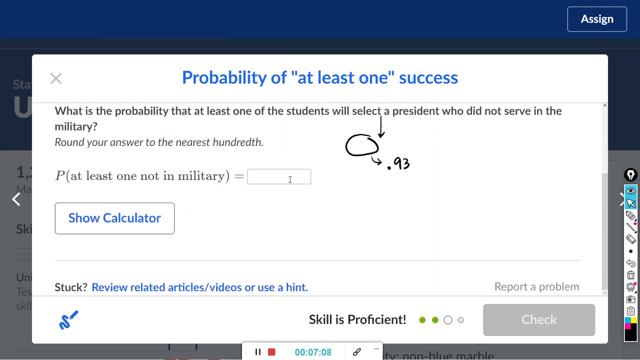 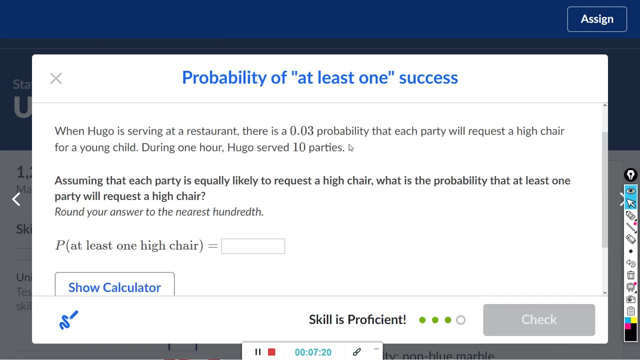 When Hugo was serving at a restaurant, there was a .03 probability that each party would be serving at the same restaurant- will request a high chair for a young child. during one hour you go serve 10 parties, assuming that each party is equally likely to request a high chair. 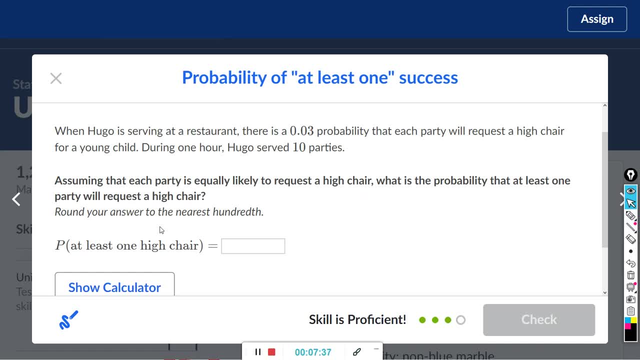 what is the probability that at least one party will request a high chair? okay, so the opposite of at least one is none. all right, so it's gonna be one, minus the probability that none request a high chair, all right. so see, when they say at least one, that can be one, two, three and so on, up to ten parties, right, so the? 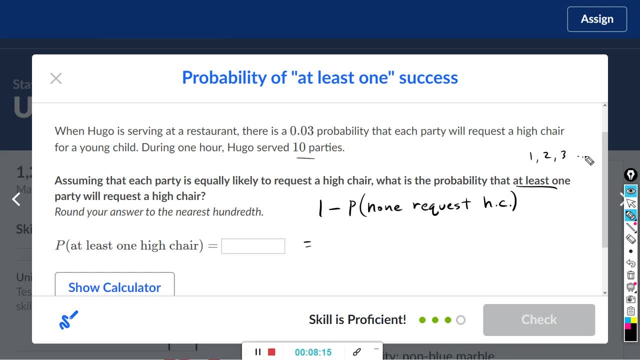 opposite of one, two, three, four, five, six, seven, eight, nine, ten. the opposite of all those is going to be none. so it's going to be one minus the probability that none selected. alright. so if, point, if the chance of selecting a high chair is .03, let me see.